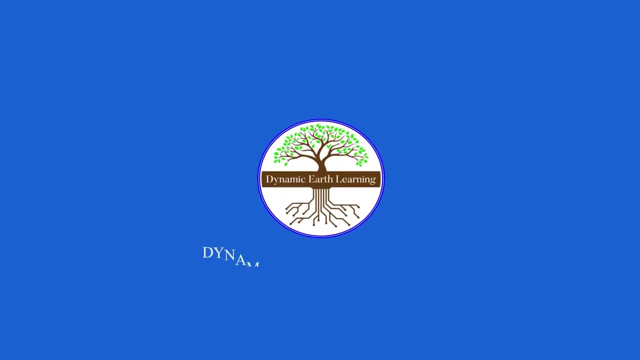 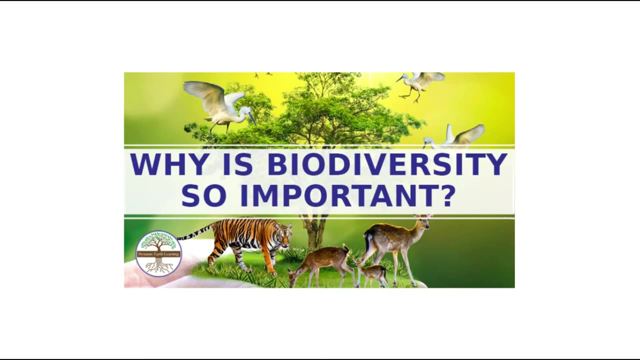 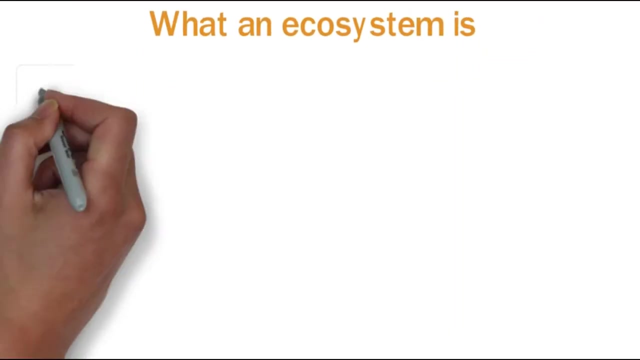 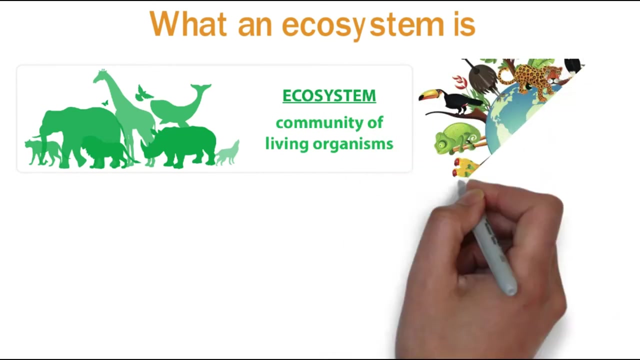 Why is biodiversity so important? To understand why biodiversity is so important, we must first understand what an ecosystem is. An ecosystem is a community of living organisms. They interact with each other in their non-living environments. For an ecosystem to function and survive, it needs 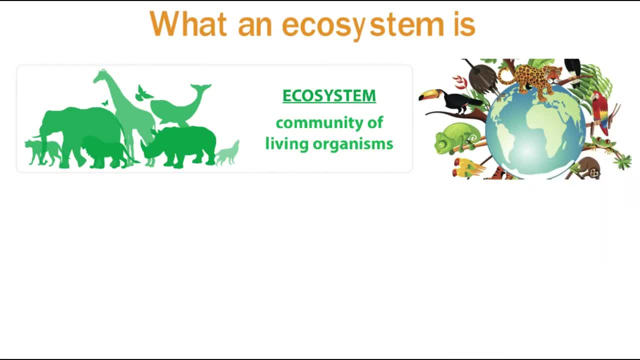 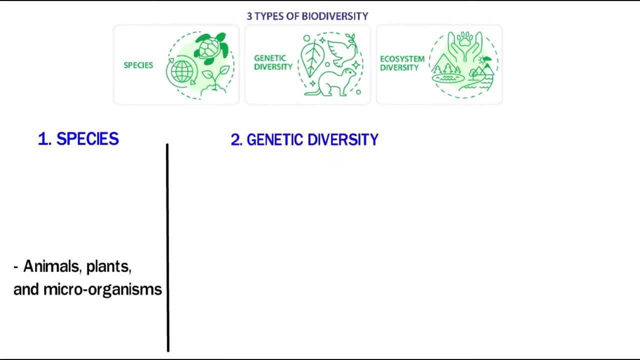 biodiversity. Biodiversity refers to the number and variety of all living things: plants, animals, insects and all living things that exist within an ecosystem. There are three types of biodiversity: Species: animals, plants and microorganisms. Genetic diversity: animals, birds, aquatic animals. 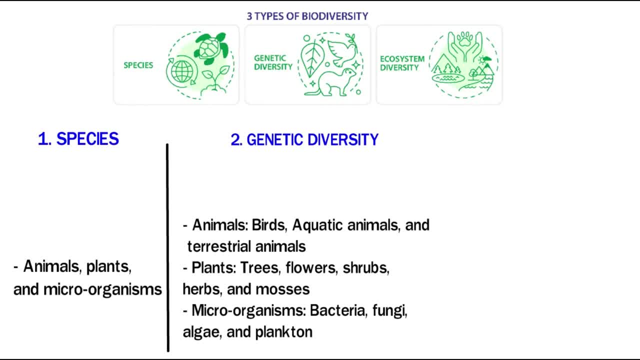 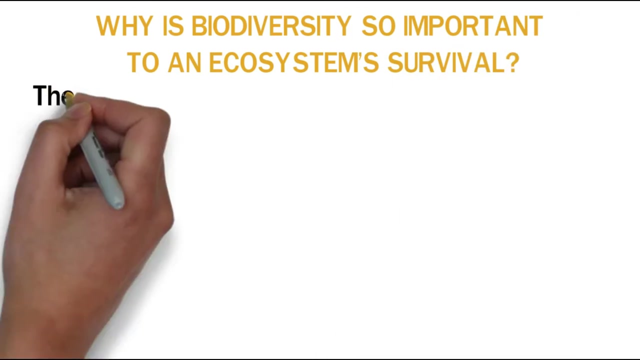 and terrestrial animals, Plants, trees, flowers, shrubs, herbs and mosses, Microorganisms, bacteria, fungi, algae and plankton. Ecosystem diversity, Forest ecosystems, Grassland ecosystems, Desert ecosystems, Aquatic ecosystems. Why is biodiversity so important to an ecosystem's survival? The circle of life. Life depends on life. 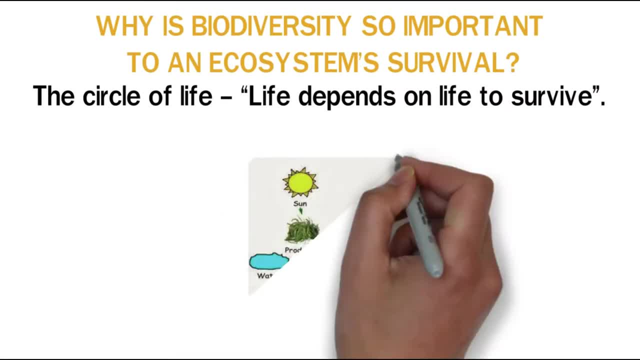 to survive. All living species are interconnected and need each other to survive. For example, plants feed on soil, Insects feed on plants and, in return, pollinate plants, helping them to spread and bear fruit. Birds eat the fruit, helping new plants to grow by dropping seeds. Birds die and 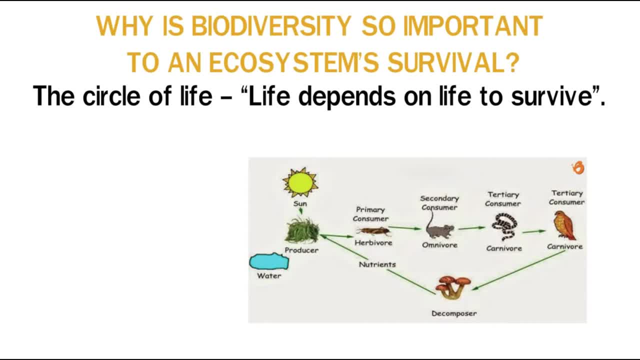 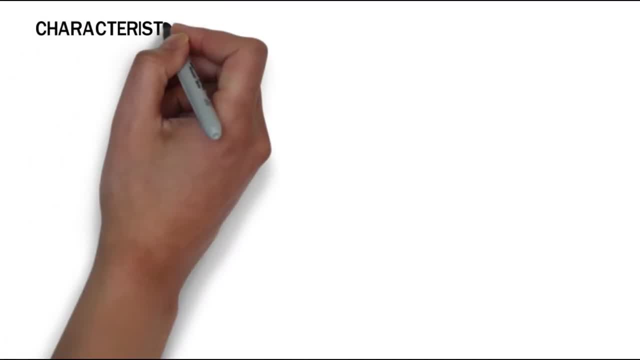 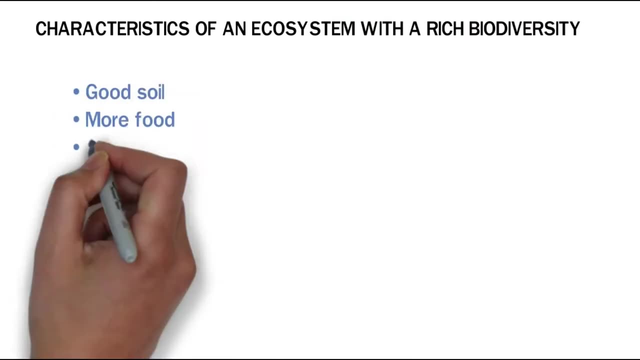 microorganisms feed on them. Microorganisms then release nutrients into the soil. Nutrients then feed the plants and the circle of life is complete Characteristics of an ecosystem with a rich biodiversity. Areas with rich biodiversity have good soil, more food, cleaner air, cleaner water. 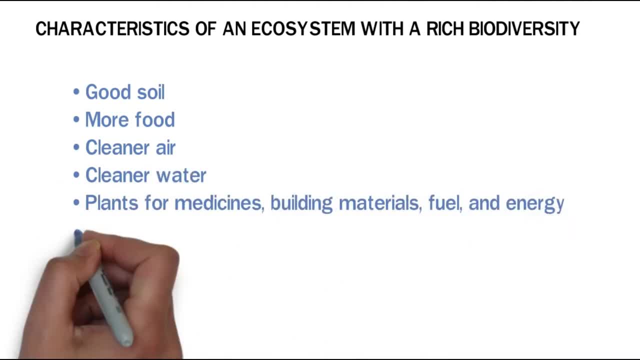 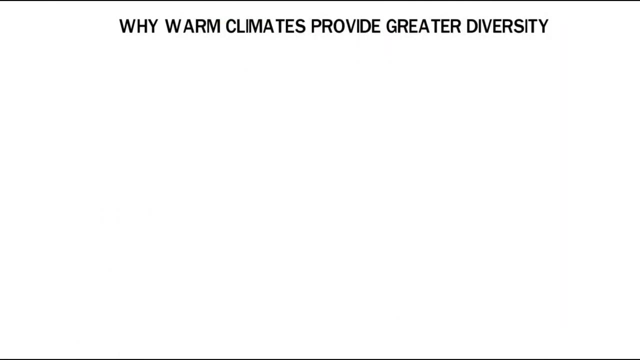 plants, for medicines, building materials, fuel and energy, minerals, less harmful pests and diseases. All these factors offer humans social, economic, cultural and ecological benefits. Why warm climates provide greater diversity? In certain parts of the globe, you will find greater biodiversity than others. 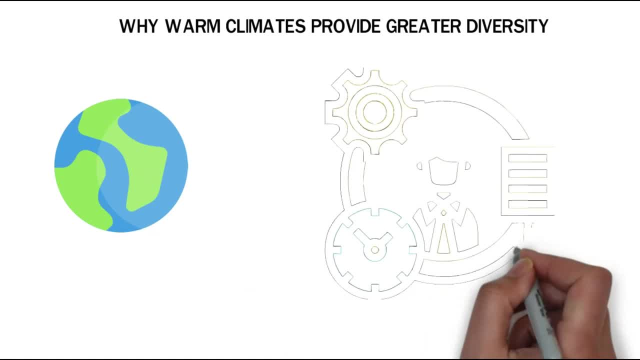 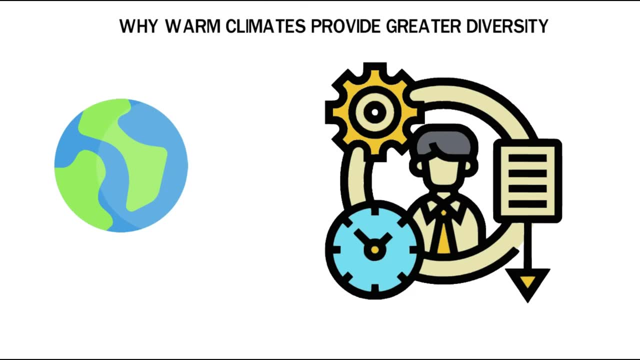 An international study done by a team of scientists shows temperature drives biodiversity. Data revealed that more plant species can grow in warm temperatures. That means more food and types of food for animals. This, in turn, will increase biodiversity, And that's why we're. 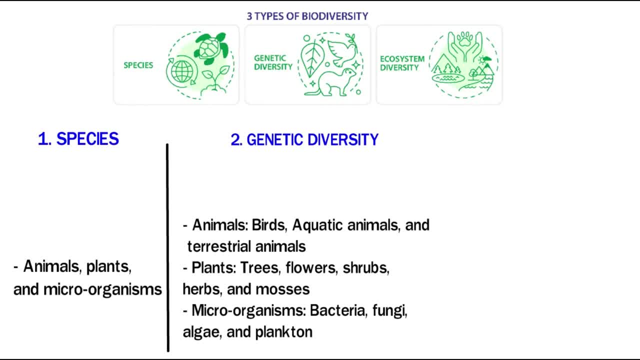 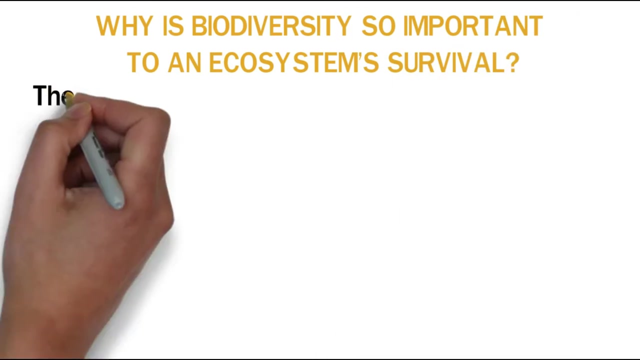 and terrestrial animals, Plants, trees, flowers, shrubs, herbs and mosses, Microorganisms, bacteria, fungi, algae and plankton. Ecosystem diversity, Forest ecosystems, Grassland ecosystems, Desert ecosystems, Aquatic ecosystems. Why is biodiversity so important to an ecosystem's survival? The circle of life. Life depends on life. 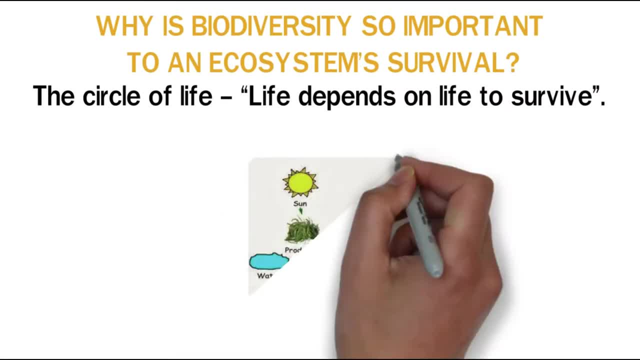 to survive. All living species are interconnected and need each other to survive. For example, plants feed on soil, Insects feed on plants and, in return, pollinate plants, helping them to spread and bear fruit. Birds eat the fruit, helping new plants to grow by dropping seeds. Birds die and 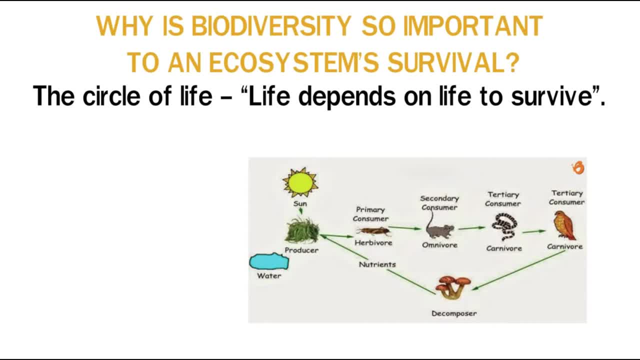 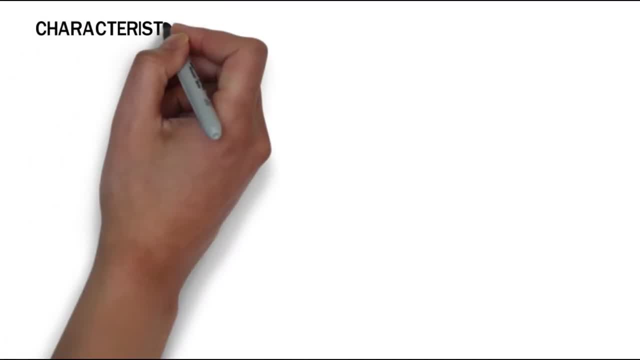 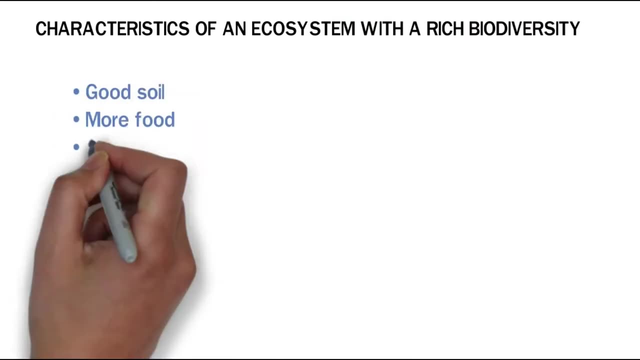 microorganisms feed on them. Microorganisms then release nutrients into the soil. Nutrients then feed the plants and the circle of life is complete Characteristics of an ecosystem with a rich biodiversity. Areas with rich biodiversity have good soil, more food, cleaner air, cleaner water. 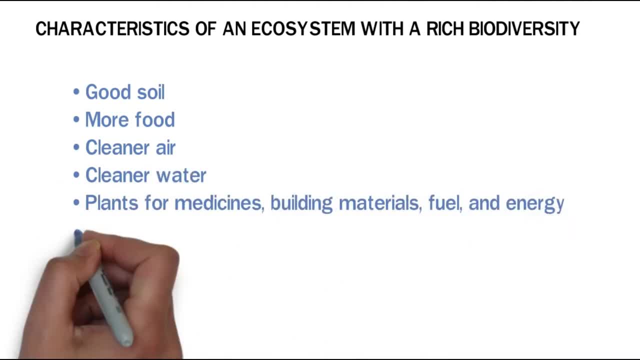 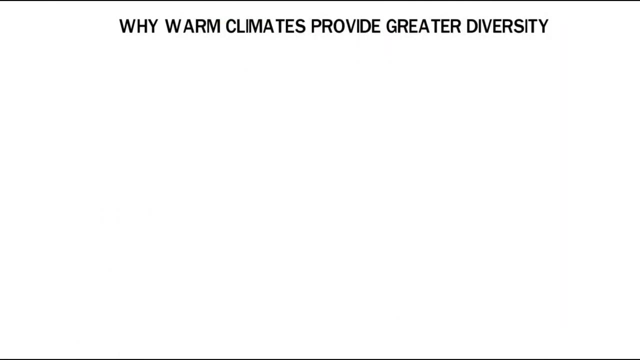 plants, for medicines, building materials, fuel and energy, minerals, less harmful pests and diseases. All these factors offer humans social, economic, cultural and ecological benefits. Why warm climates provide greater diversity? In certain parts of the globe, you will find greater biodiversity than others. 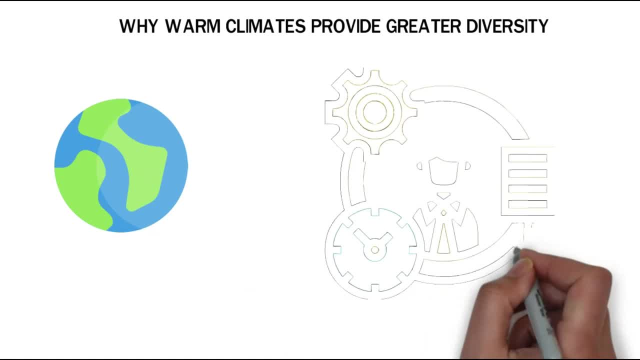 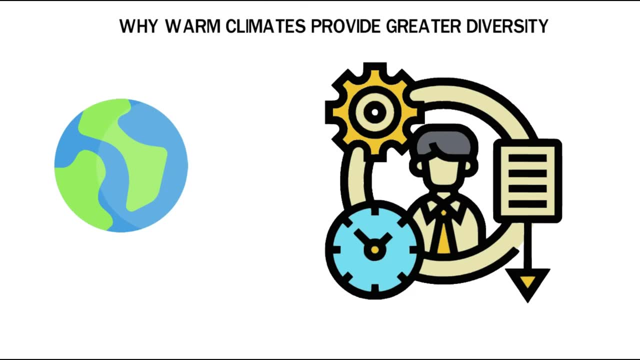 An international study done by a team of scientists shows temperature drives biodiversity. Data revealed that more plant species can grow in warm temperatures. That means more food and types of food for animals. This, in turn, will increase biodiversity, And that's why we're. 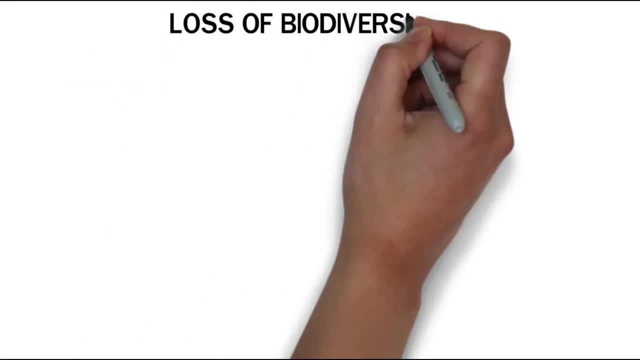 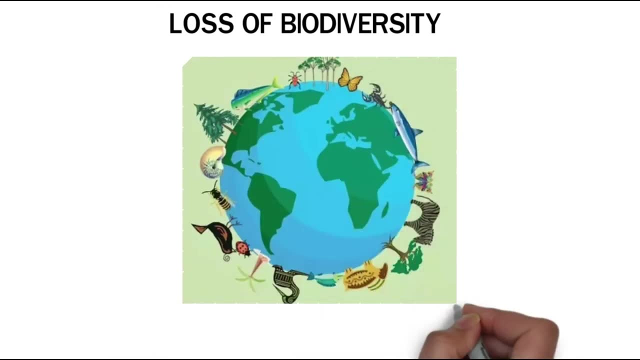 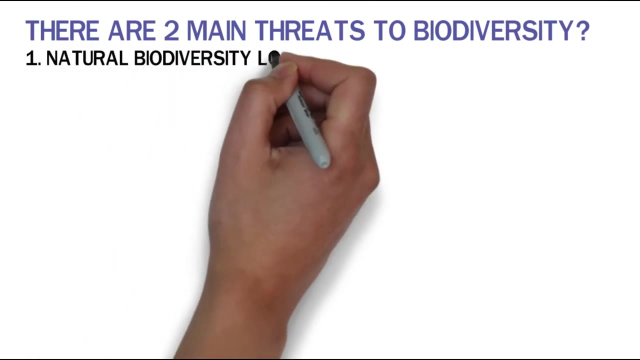 going to talk about biodiversity in the future. The effects of biodiversity loss can have dramatic effects on an ecosystem. The smallest decrease in biodiversity disrupts the balance of an ecosystem. There are two main threats to biodiversity: Natural biodiversity loss. Seasons At the equator, where climates are steady. 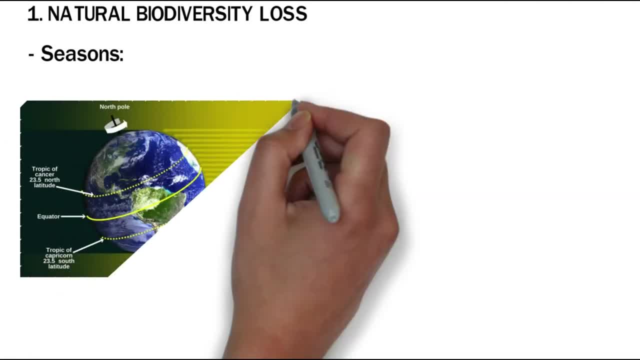 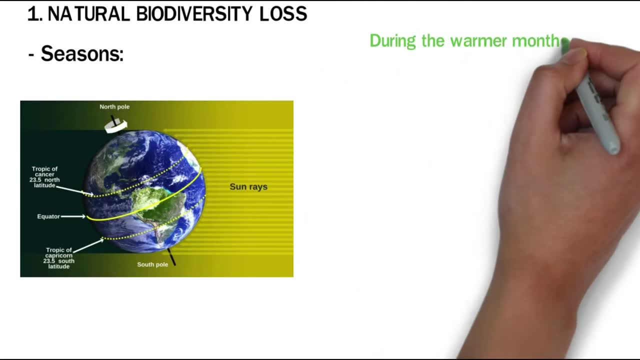 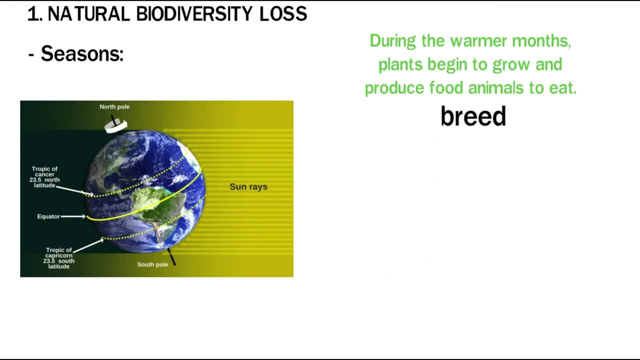 you have small seasonal changes. Natural cycles cause changes in temperature and rainfall. These changes affect the rise and fall of biodiversity. During the warmer months, plants begin to grow and produce food animals to eat. In turn, these animals breed, causing the area's biodiversity to rise. 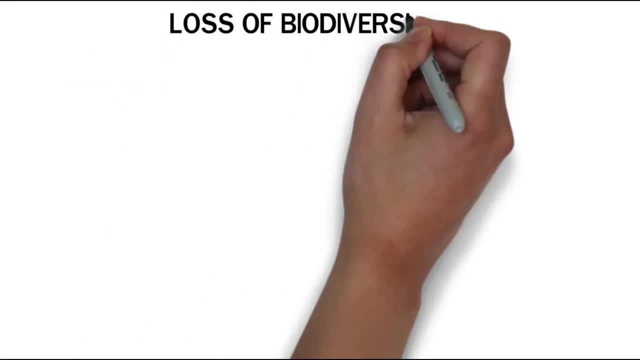 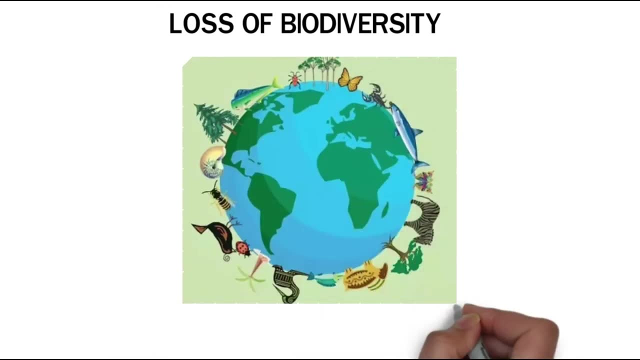 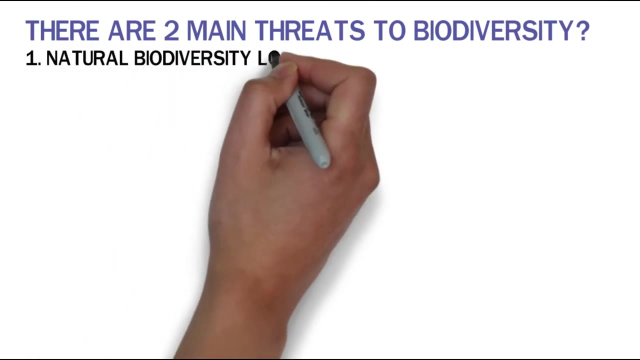 going to talk about biodiversity in the future. The effects of biodiversity loss can have dramatic effects on an ecosystem. The smallest decrease in biodiversity disrupts the balance of an ecosystem. There are two main threats to biodiversity: Natural biodiversity loss. Seasons At the equator, where climates are steady. 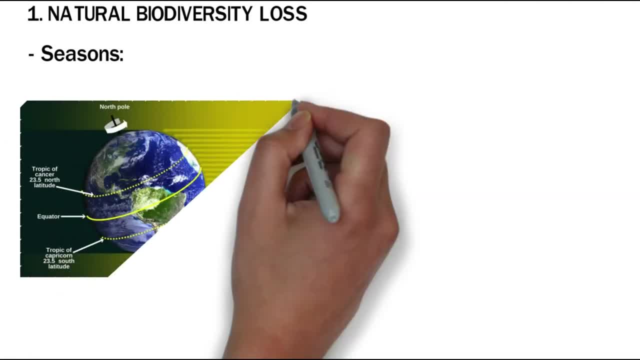 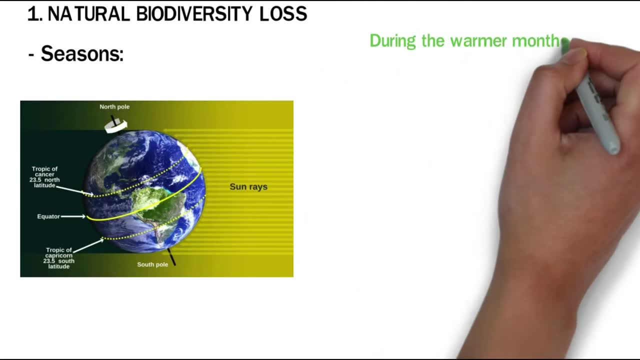 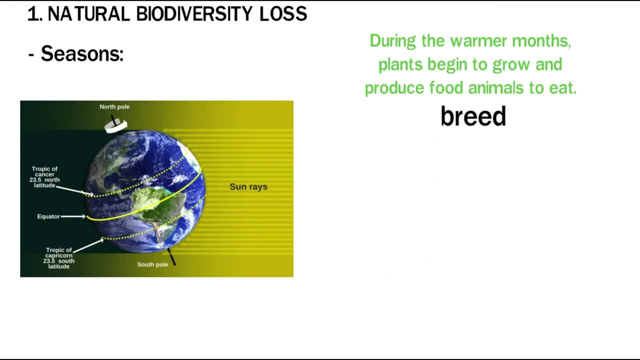 you have small seasonal changes. Natural cycles cause changes in temperature and rainfall. These changes affect the rise and fall of biodiversity. During the warmer months, plants begin to grow and produce food animals to eat. In turn, these animals breed, causing the area's biodiversity to rise. 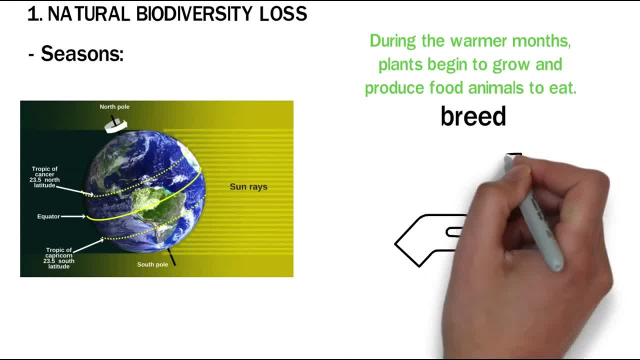 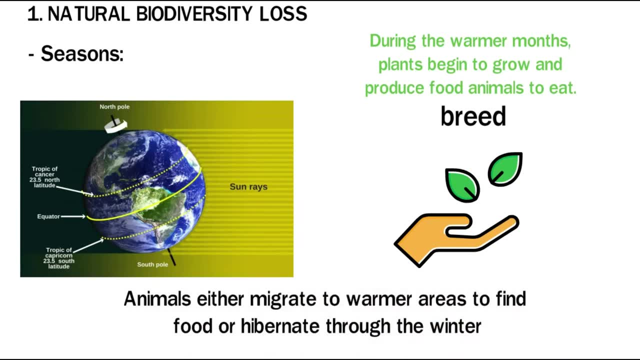 The opposite happens. during the colder months, Plants stop growing and producing food, Insects begin to die out. Animals either migrate to warmer areas to find food or hibernate through the winter, Because they rise and fall every year. this kind of natural biodiversity loss is sustainable. 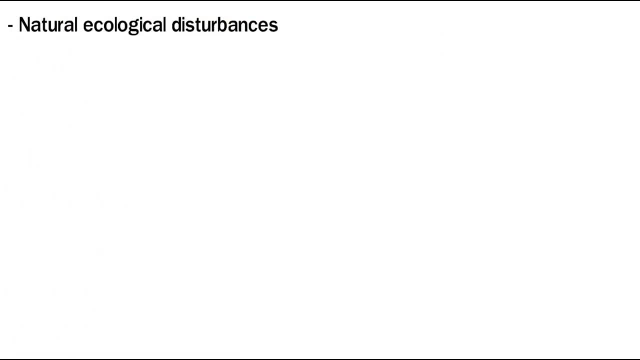 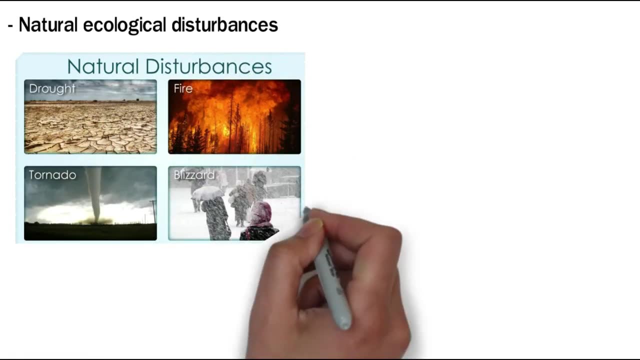 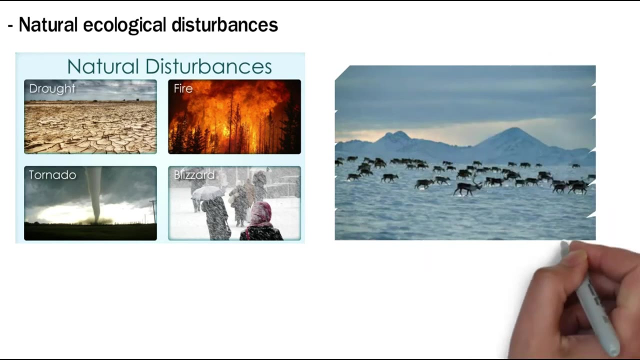 Natural ecological disturbances. Nature is always changing. Earthquakes, floods, hurricanes and wildfires all have an effect on biodiversity loss. In areas affected by natural ecological disturbances, species have to migrate, searching for new homes and food. These disturbances are temporary. 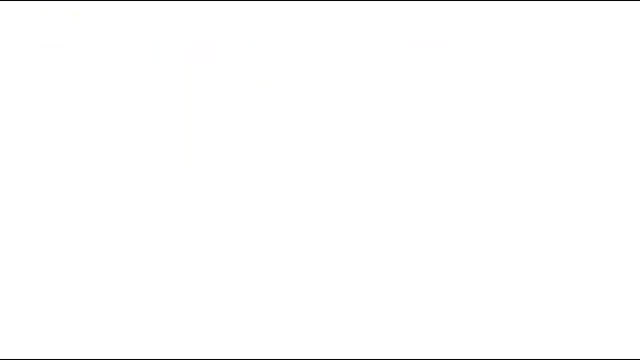 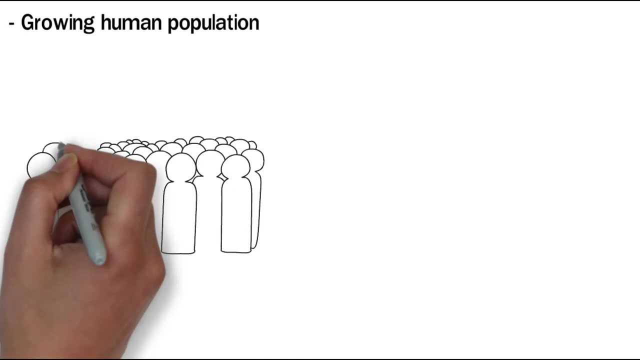 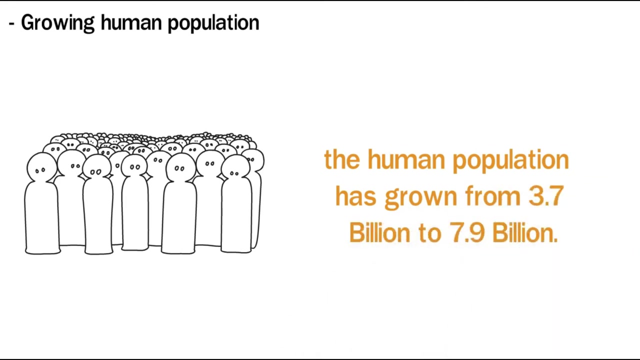 The ecosystem will adapt and return to the affected area. Human-driven biodiversity loss. Humans are the biggest threat to biodiversity loss and these disturbances caused by humans have a lasting impact. They destroy ecosystems and biodiversity. Growing human population. Between 1970 and 2021, the human population has grown from 3.7 billion to 7.9 billion. 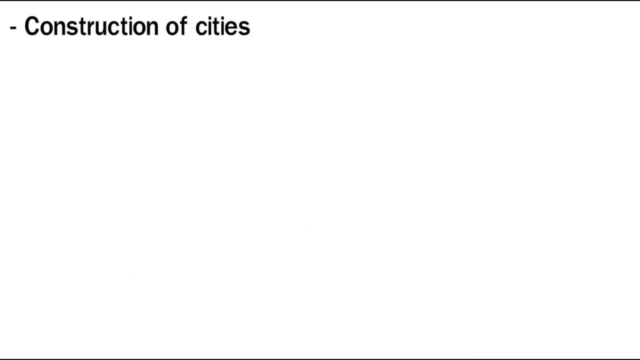 Construction of cities. With this rise in the world's population, more and more space is needed. Cities and houses are built for the booming population. Farming: More and more land is needed to grow food to sustain the growing population. Over 40% of the world's habitable land has been converted for agricultural purposes. 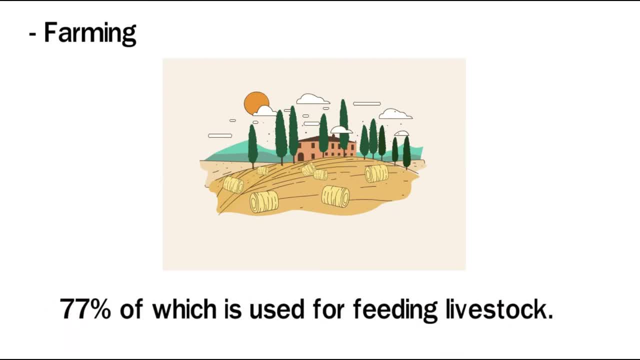 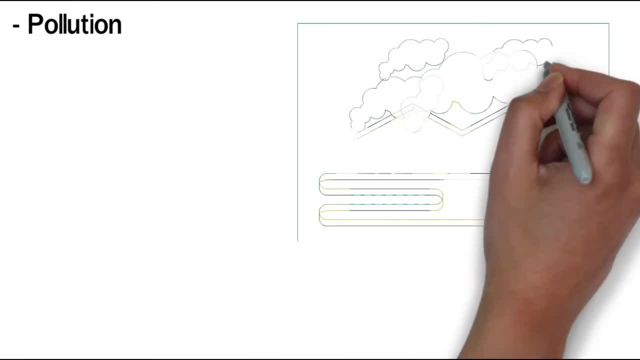 77% of which is used for feeding livestock Pollution. A growth in population equals a rise in consumption, which leads to a rise in waste produced. Waste pollutes and destroys the ecosystems around us through plastics and chemicals. It also takes up space. 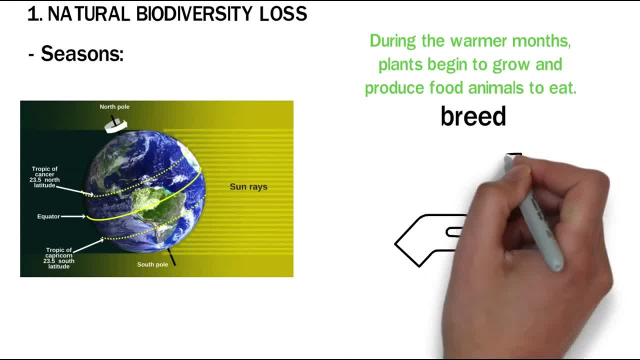 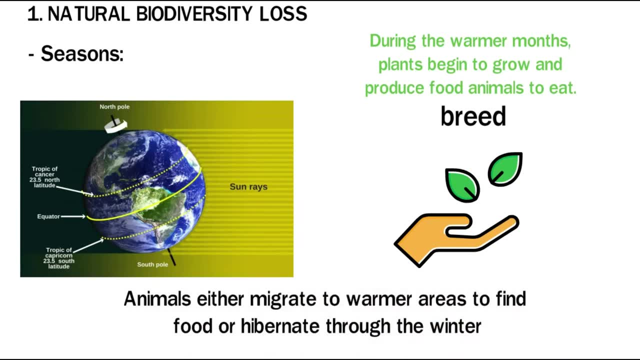 The opposite happens. during the colder months, Plants stop growing and producing food, Insects begin to die out. Animals either migrate to warmer areas to find food or hibernate through the winter, Because they rise and fall every year. this kind of natural biodiversity loss is sustainable. 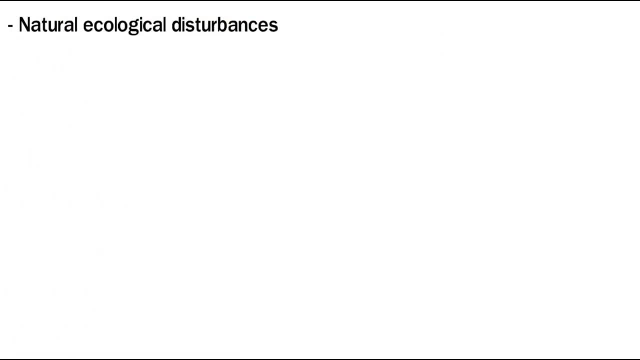 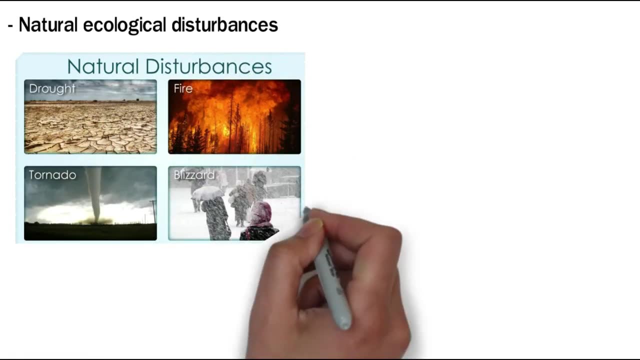 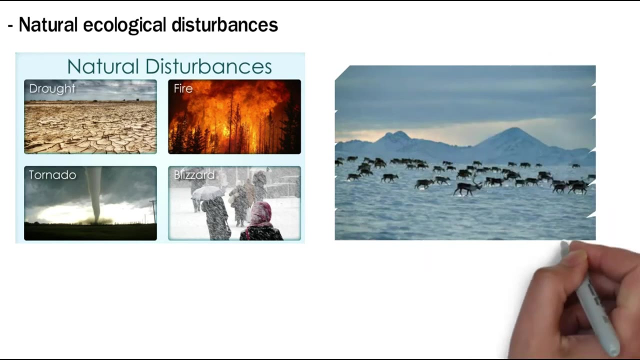 Natural ecological disturbances. Nature is always changing. Earthquakes, floods, hurricanes and wildfires all have an effect on biodiversity loss. In areas affected by natural ecological disturbances, species have to migrate, searching for new homes and food. These disturbances are temporary. 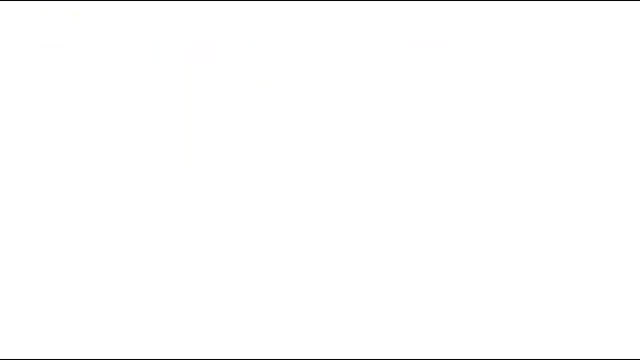 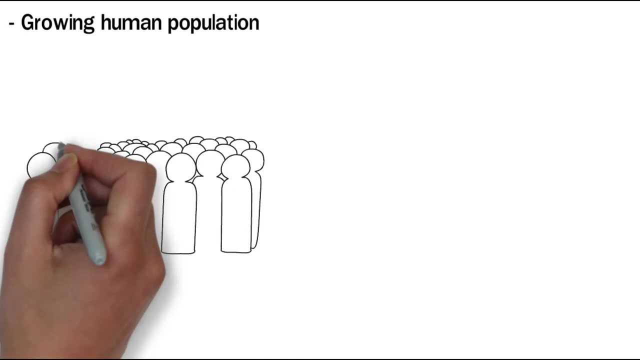 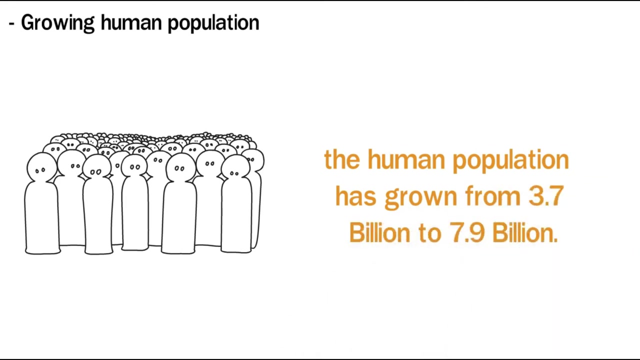 The ecosystem will adapt and return to the affected area. Human-driven biodiversity loss. Humans are the biggest threat to biodiversity loss and these disturbances caused by humans have a lasting impact. They destroy ecosystems and biodiversity. Growing human population. Between 1970 and 2021, the human population has grown from 3.7 billion to 7.9 billion. 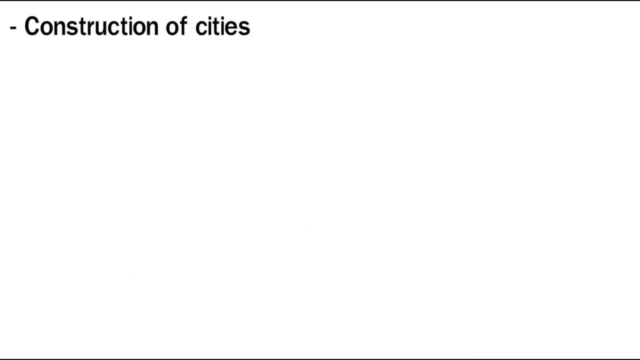 Construction of cities. With this rise in the world's population, more and more space is needed. Cities and houses are built for the booming population. Farming: More and more land is needed to grow food to sustain the growing population. Over 40% of the world's habitable land has been converted for agricultural purposes. 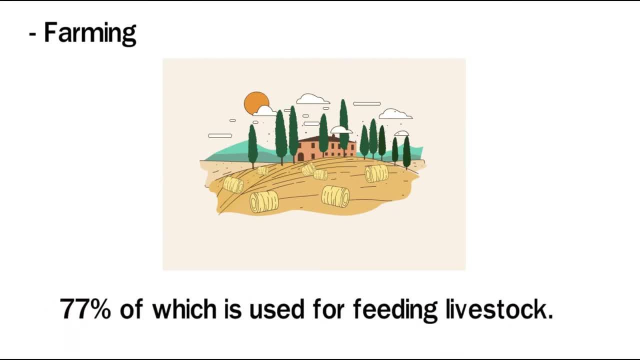 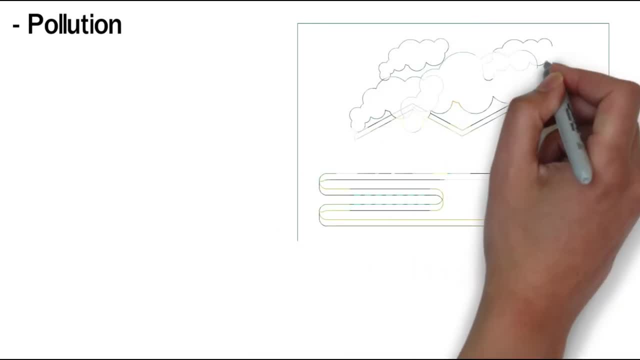 77% of which is used for feeding livestock Pollution. A growth in population equals a rise in consumption, which leads to a rise in waste produced. Waste pollutes and destroys the ecosystems around us through plastics and chemicals. It also takes up space. 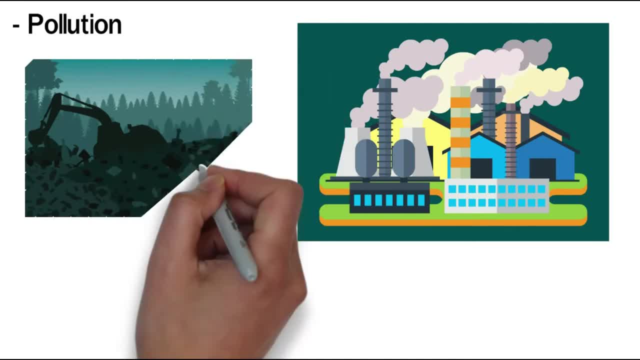 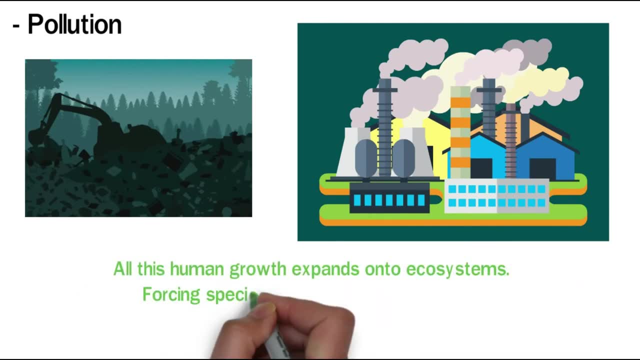 Stretches of land must be cleared to create landfills. All the waste produced by human consumption is dumped here. All this human growth expands onto ecosystems, forcing species out of the natural habitats or wiping them out. All this human growth expands onto ecosystems, forcing species out of the natural habitats or wiping them out. 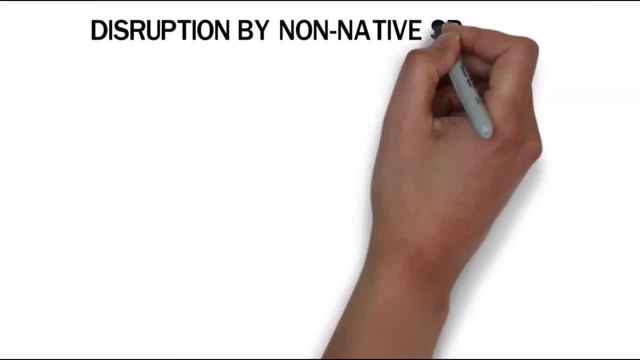 All this human growth expands onto ecosystems, forcing species out of the natural habitats or wiping them out completely. All this human growth expands onto ecosystems, forcing species out of the natural habitats or wiping them out completely. Disruption by non-native species: There is a less common but growing threat to biodiversity. 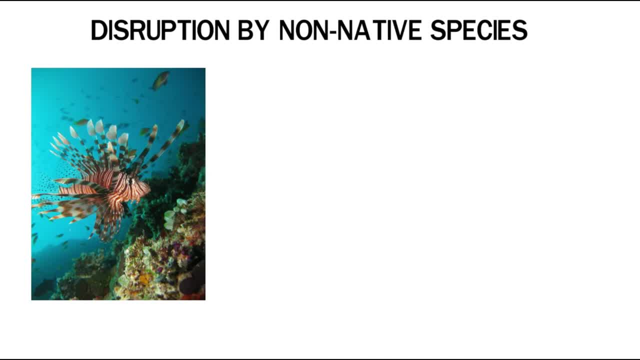 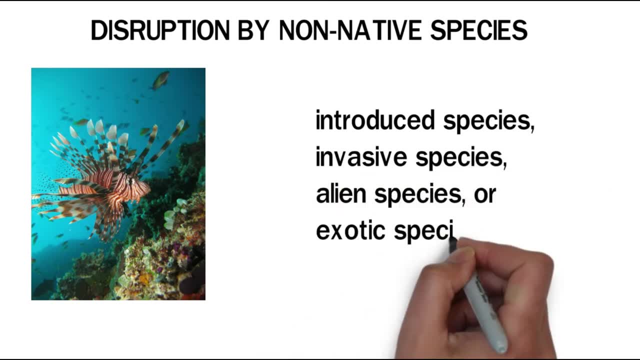 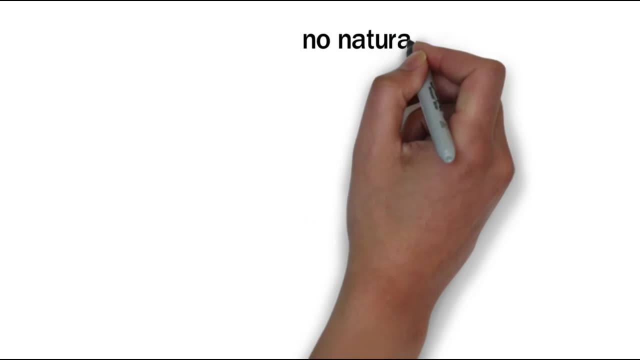 The disruption of ecosystems by non-native species, Also known as introduced species, invasive species, alien species or exotic species. These are species that have been brought into an ecosystem either by humans or have migrated from other areas. Because these species are not native to their new area, they often have no natural predators. 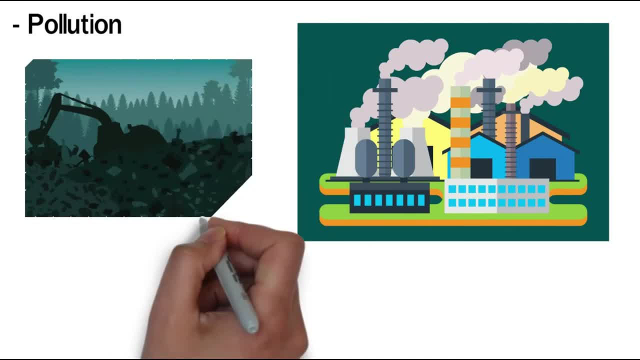 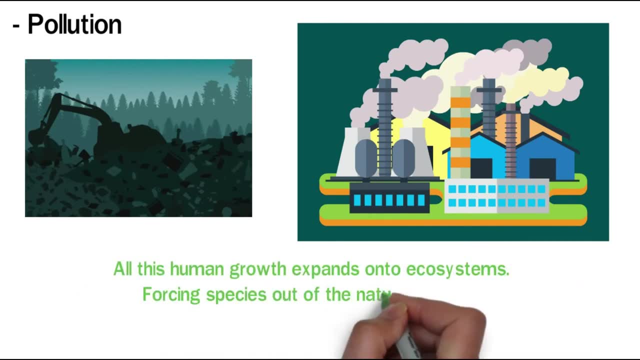 Stretches of land must be cleared to create landfills. All the waste produced by human consumption is dumped here. All this human growth expands onto ecosystems, forcing species out of the natural habitats or wiping them out of the natural habitat. Disruption by non-native species. 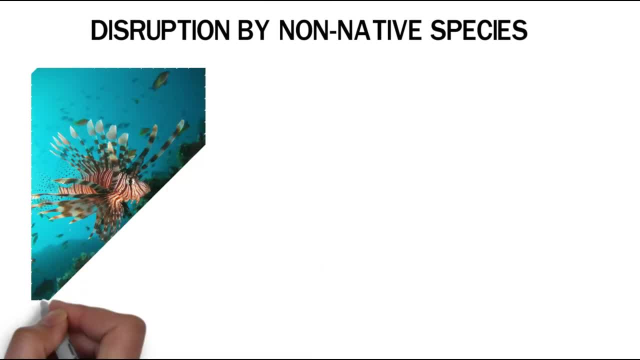 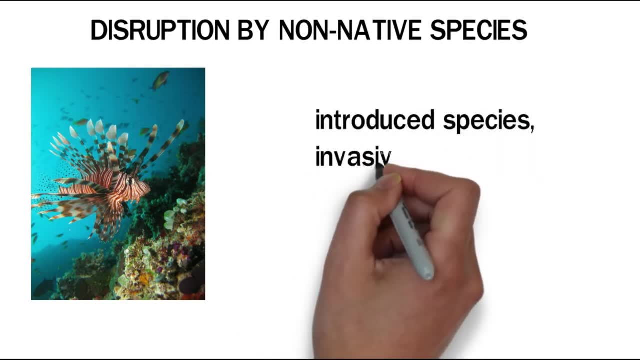 There is a less common but growing threat to biodiversity: The disruption of ecosystems by non-native species, Also known as introduced species, invasive species, alien species or exotic species. These are species that have been brought into an ecosystem either by humans or have migrated. 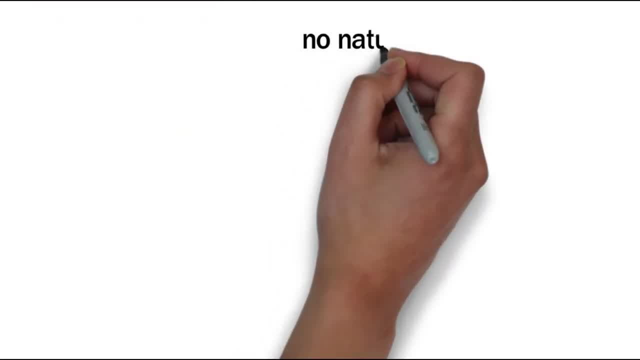 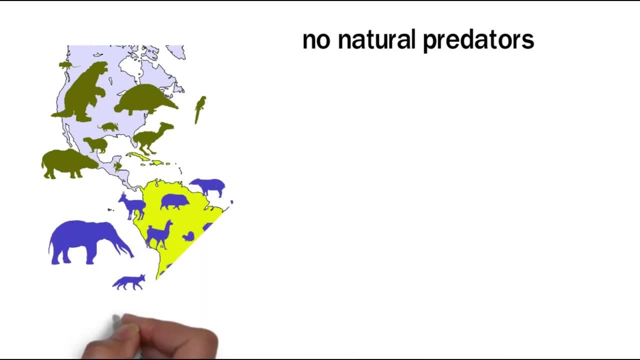 from other areas. Because these species are not native to their new area, they often have no natural predators. Natural predators keep their population in balance. Non-native species can become overpopulated, eating local crops too quickly for them to grow back in natural and sustainable cycles. This goes for plants as well. Non-native plants may grow much faster in a climate they are not used to stealing. all the soil, nutrients and sunlight native plants need to grow. Other non-native species can become the predator in an ecosystem, wiping out local animals. 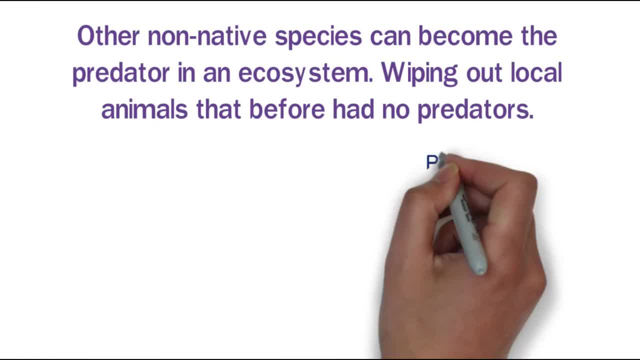 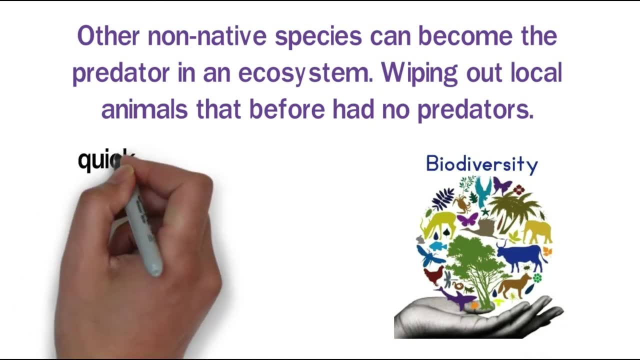 that before had no predators. Some ecosystems are not equipped to sustain such predators. The loss of biodiversity can be a problem. The loss of biodiversity may begin with the loss of one species, then quickly lead to more and more species will die out or migrate, either for food or safety. Where do you find the greatest amount of biodiversity? Amazonia. In the warm tropical rainforests of South America lies Amazonia. It holds the greatest amount of biodiversity. It is an area so large that it covers eight countries. How does loss of biodiversity affect humans? 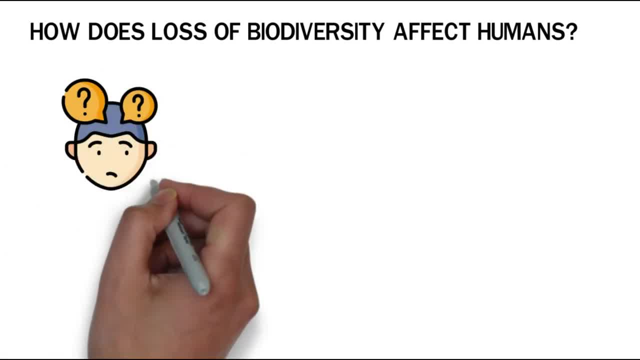 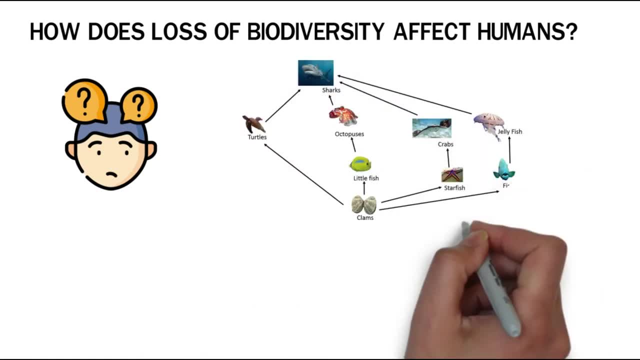 The answer to that question is scary. An ecosystem is like a chain. It is a chain kept together by links. Destroy one link and you destroy the whole chain. Planet Earth is an ecosystem filled with smaller ecosystems surviving off of biodiversity. 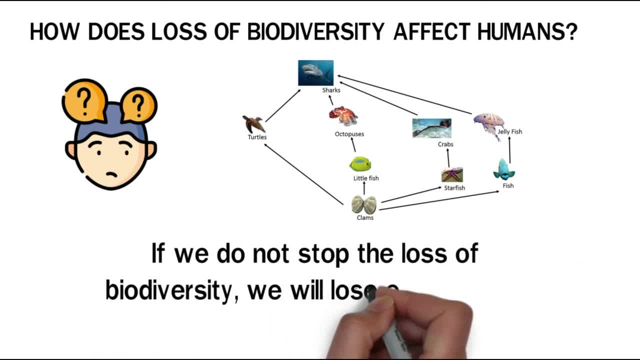 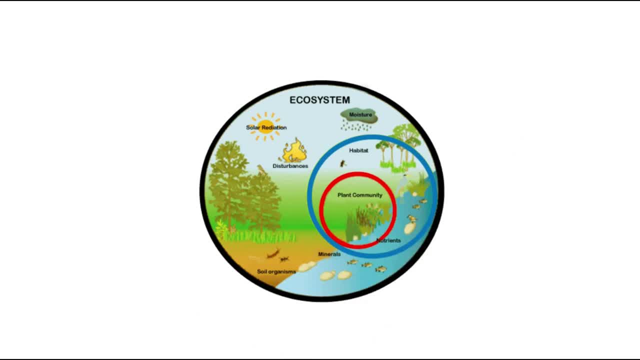 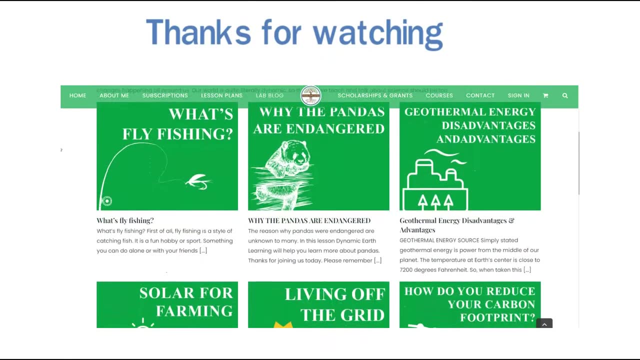 If we do not stop the loss of biodiversity, we will lose ecosystems One by one. the ecosystems around the planet will have no biodiversity, nothing to sustain themselves and, unfortunately, will fail us all. Thanks for watching. Remember to check out our blog and online short courses in the description below for 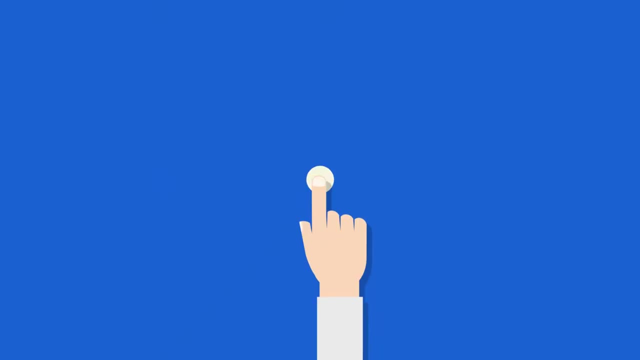 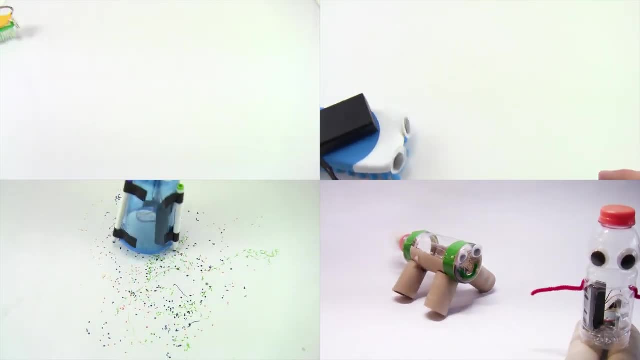 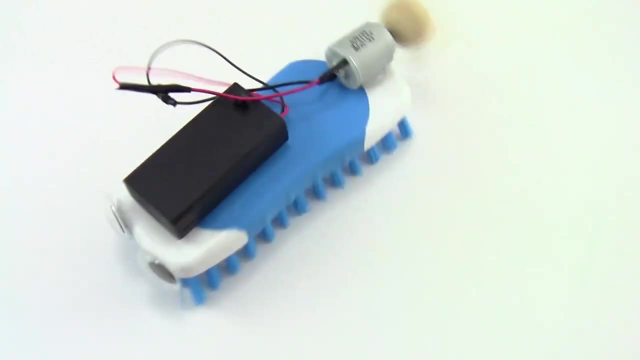 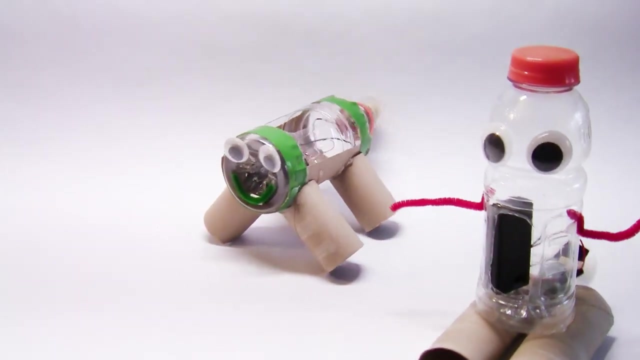 The Science Buddies Bristlebot Kit lets you build four different robots from household items: A tiny bristlebot on the head of a toothbrush, its big cousin the brush bot, an art bot that creates art as it moves, and a junk bot made from recycled materials.